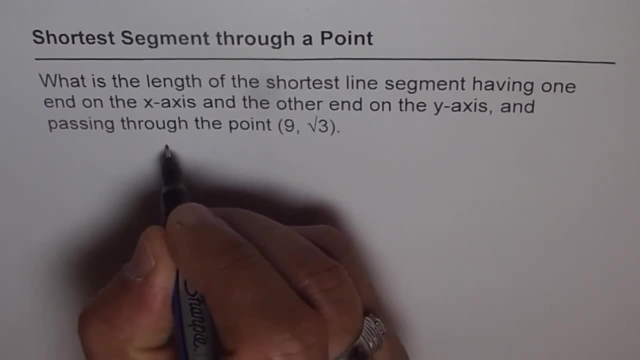 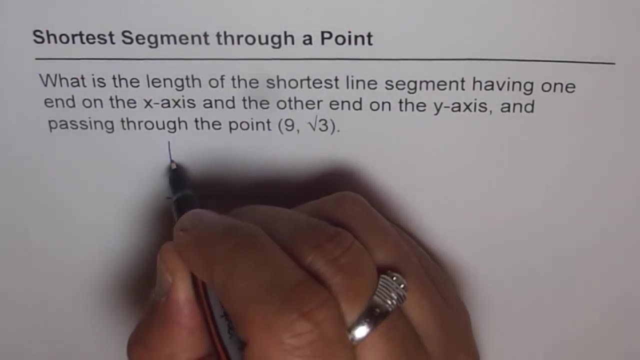 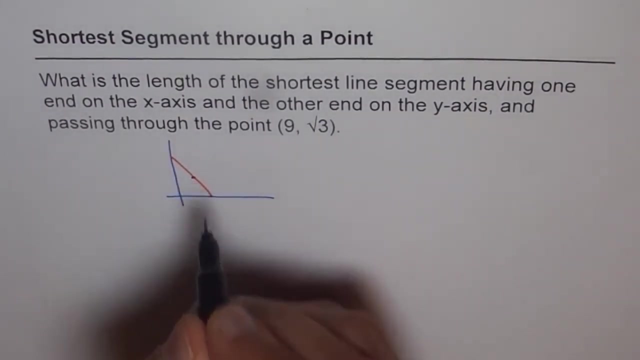 point 9, square root 3.. So let's sketch this out here and then try to figure out how to do this question. So let's say: this is our coordinate system and that's the shortest line segment we are talking about. And here let's consider that we have a point here which 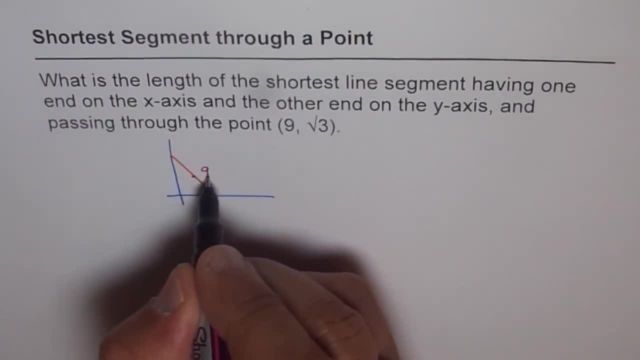 is 9 square root 3.. So if this point is 9 square root 3, it really means that if I drop a perpendicular from here, it is 9 units from 0 and square root 3 is the vertical Correct. That is what it is. And let us assume that if I have a but and then I have a square root 3, this is what I want to do. So let's say that we have the same line segment, we have the same line segment And here we have 9 square root 3, and this is the same line segment. Now, how do we do this? 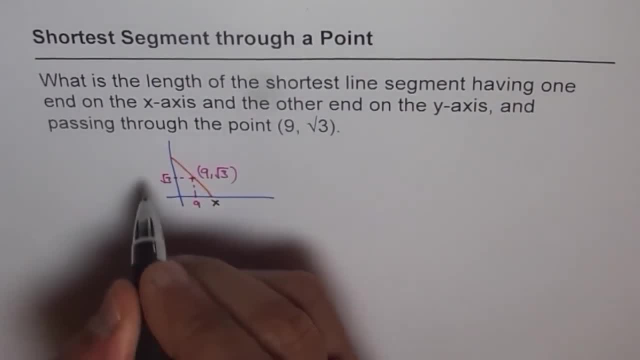 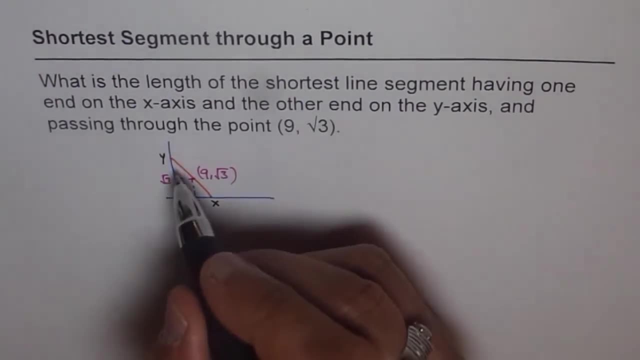 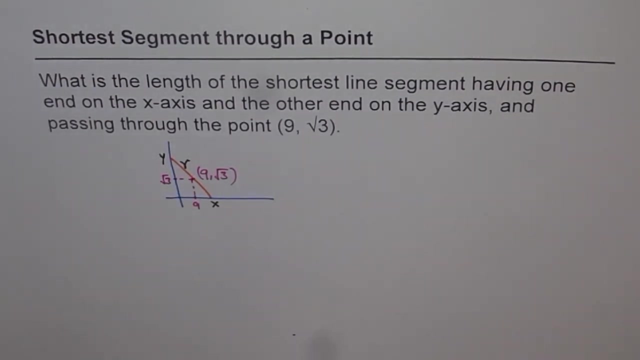 that x and y intercepts are at x and y respectively, then what we are supposed to find is the shortest length of this segment. let this be r, correct? so this r is equals to x square plus y square. but then x and y are two different variables. we need to relate them somehow. so to relate them. 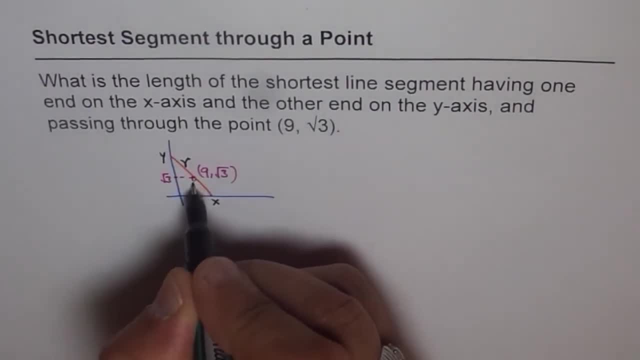 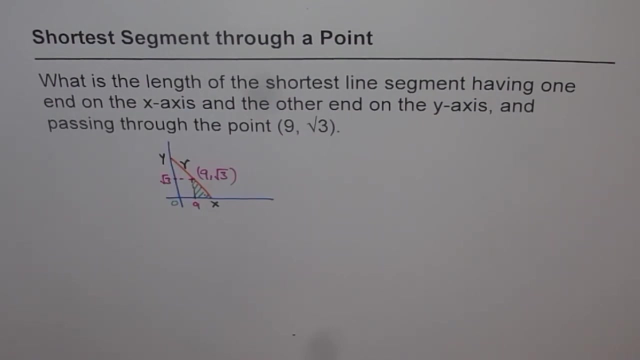 what we can do is we can consider these two triangles. that means this small triangle and the big triangle, right with the origin. they are 90 degrees each and that angle is common. so these two triangles are similar. now, since they are similar, their ratios are of sides are 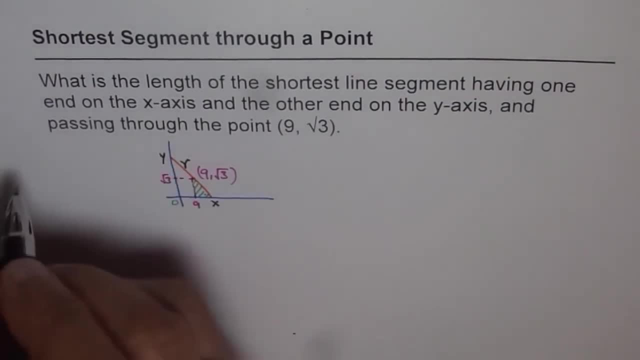 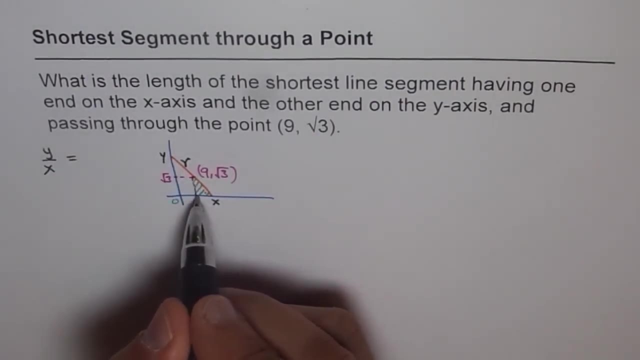 proportional. so we can say y over x, which is y over x. this over this is equals to this height, over this length. now, this height is square root three. we know that. now, what is that small length? that small length is x minus 9, correct, so I can write this as x minus 9. but this ratio of similar triangles help us to. 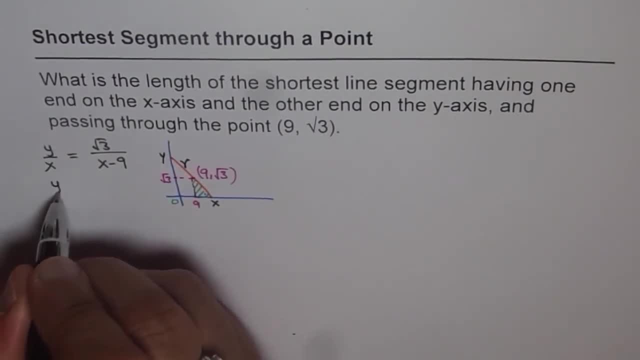 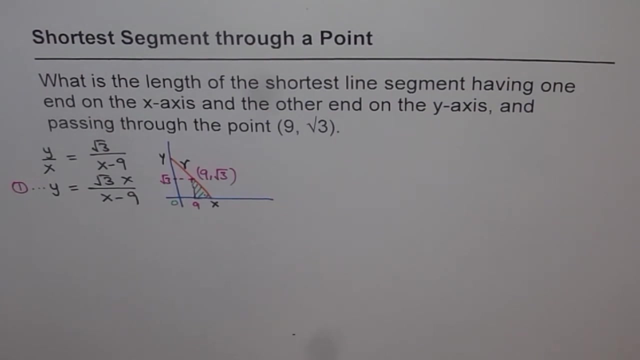 relate y with x. so we can write now: y equals to square root 3x over x minus 9. now this relation will give it a number and let's say this is our equation number 1.. Now let us also find dy dx from here. So dy dx will be: dy dx will be equals. 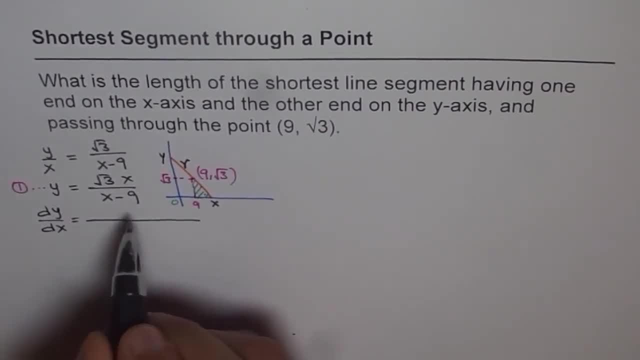 to, we will use quotient rule. So quotient rule means denominator: square x minus 9, square numerator. So we have derivative of this which is square root 3 times x minus 9, right minus derivative of this which is 1 times square root 3x. 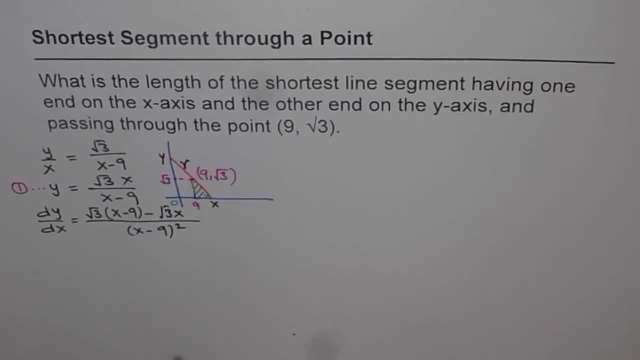 So that becomes our numerator. Now we can simplify this at this stage and we can write this as equal to square root 3x and square root 3x. cancel out. We get minus 9 times square root 3 in the numerator, minus 9 times square root 3 divided by. 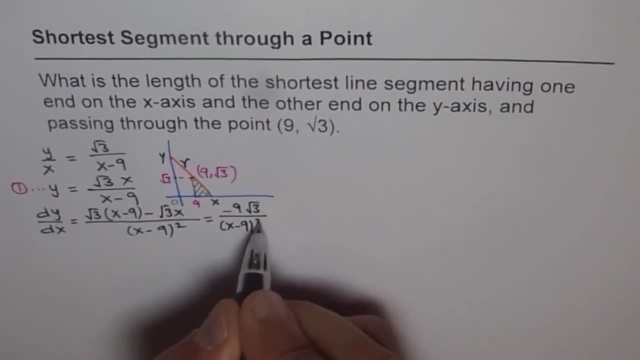 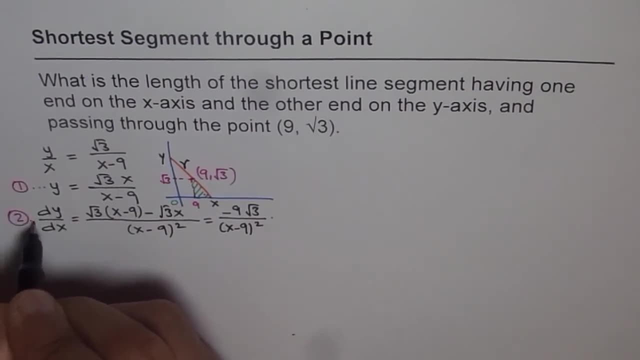 x minus 9, whole square. Well, so that is dy dx. Let me call this as equation 2.. So we now have relation of y with x and dy dx also. That is great. Now what we will do is we will relate r with x and y, So the length which we want to minimize r is actually 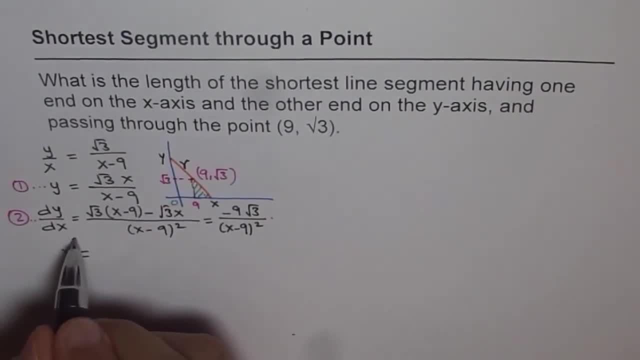 equals to, or rather we can write: r square: r square is equals to x square plus y square. right Now, that's the relation. We can differentiate with respect to x, both sides. So we get 2 times r dr dx equals to 2x plus 2 times y dy dx, So that 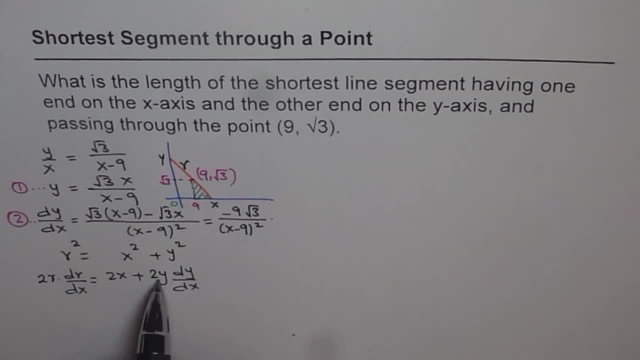 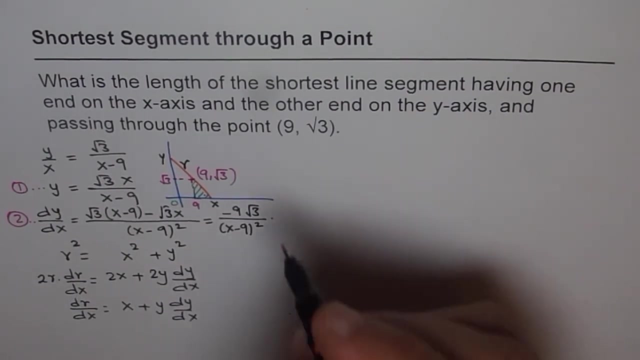 is what we get after differentiation, and we can always cancel out 2 and simplify it a bit more. So we get this dr dx as equals to x plus y dy dx correct? Now we'll take it to the right side and simplify further. 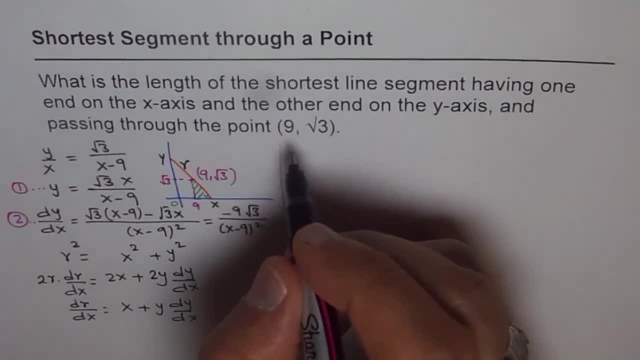 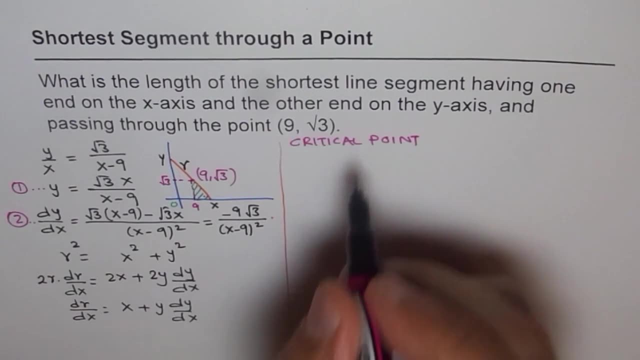 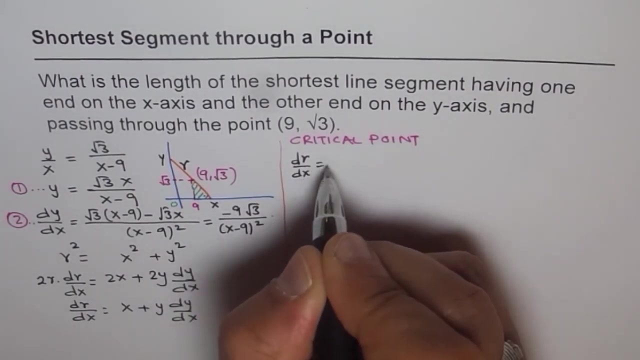 Basically, we need to find critical points. So now we'll find critical point. Now critical point is the one where dr dx should be equals to 0. So we want to put dr dx as equal to 0. That gives us a critical point. 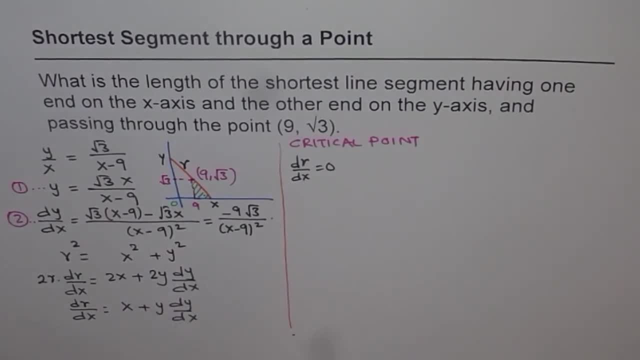 And that means x plus y over dy dx should be 0.. Now y, we know, can be written as square root 3x over x minus 9, right. And dy dx can be written as minus 9 times square root: 3 over x minus 9, whole square. 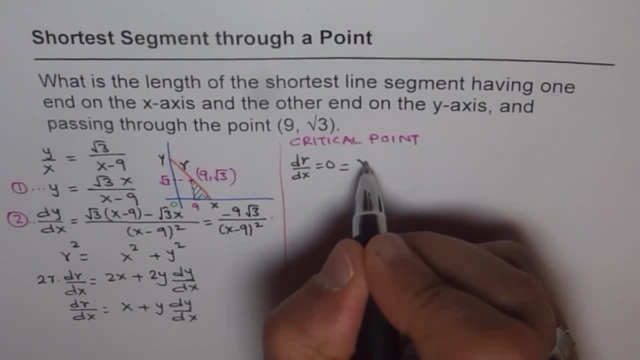 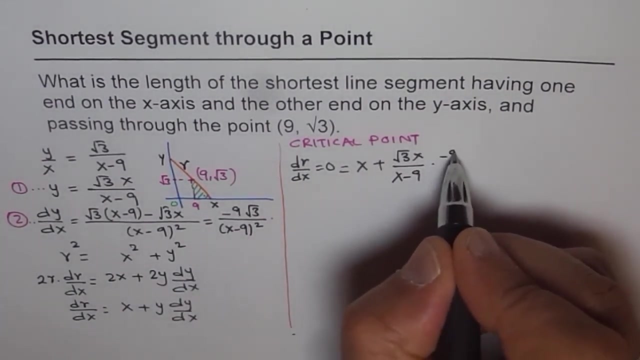 So let's write: replace x- y with those values, okay, Plus y: y is square root 3x over x minus 9, and dy- dx is minus 9 square roots. Let me put it in bracket, Otherwise it can create confusion, right. 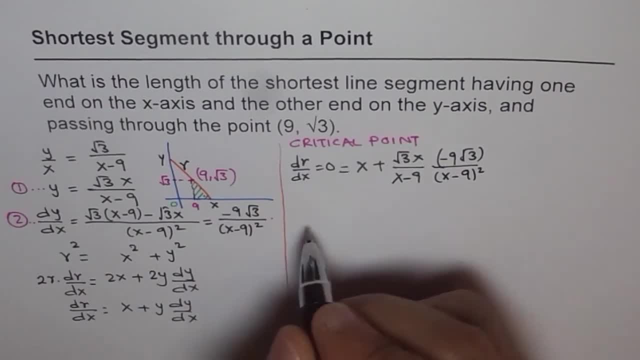 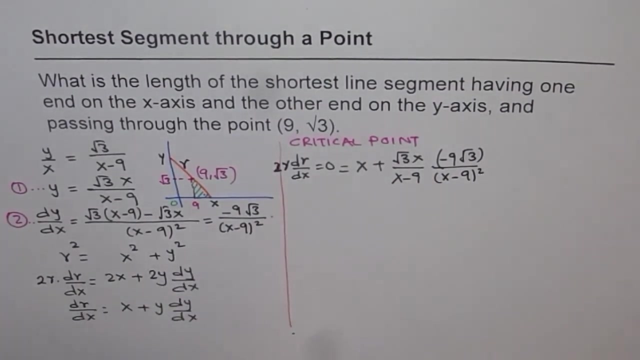 Over x minus 9, whole square right. So that is what dy dx is. So from equation 1 and 2, we got this. Now that can be simplified. Now dr dx is equals to 0. We can write even 2r, or rather r, because we cancel out 2.. 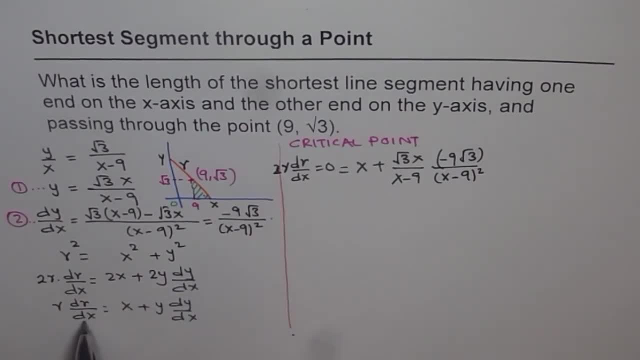 So there was r here, right? So when you equate, dr dx equals 0, r times dr dx will also be 0.. Remember that part. So this has to be equated to 0.. Let's try to simplify what we have here. 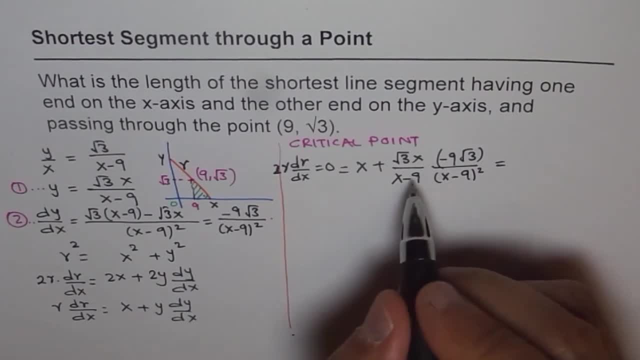 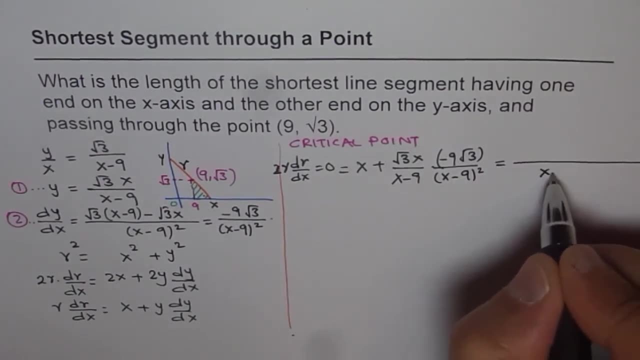 So what we can write here, as we can take x minus 9 whole cube as denominator, right? So we'll take x minus 9.. 9 whole cube, that is this denominator multiplied by x. So we get x times x minus 9 whole cube. here and there we get minus, correct? 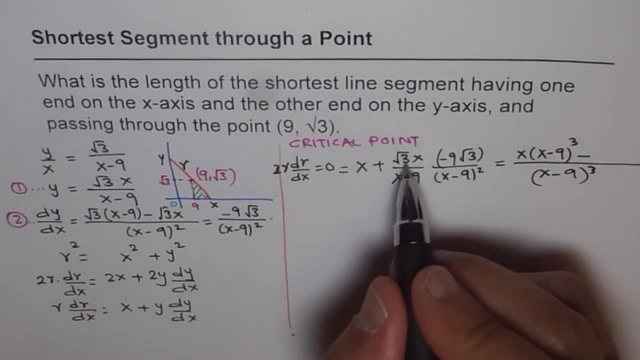 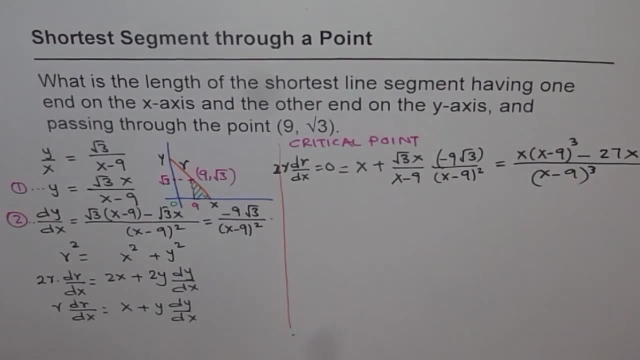 So we get minus square root 3 times square root. 3 is 3, and then 9 is 27.. So minus 27x, correct? So that is what we get in the numerator. Now for that to be 0, the numerator should be 0, correct. 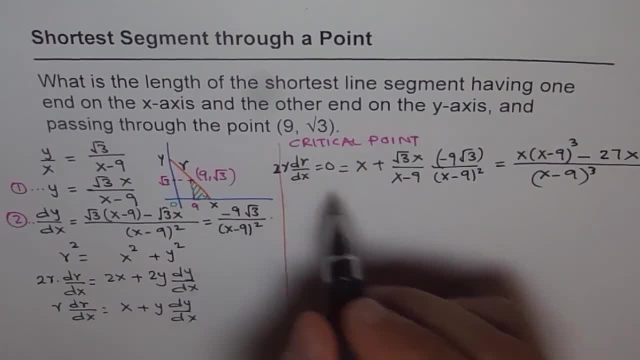 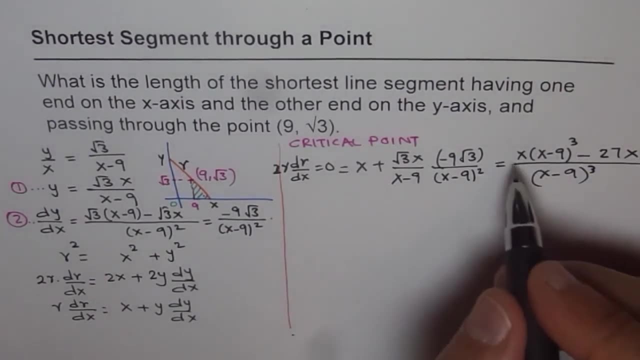 Now, that is, That is So we. So we have basically dr dx equals to this particular function. Now we can equate numerator to 0 and solve So x. we can take x times. let's take x common right. 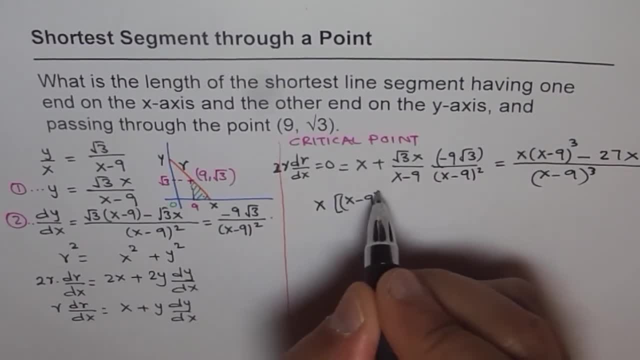 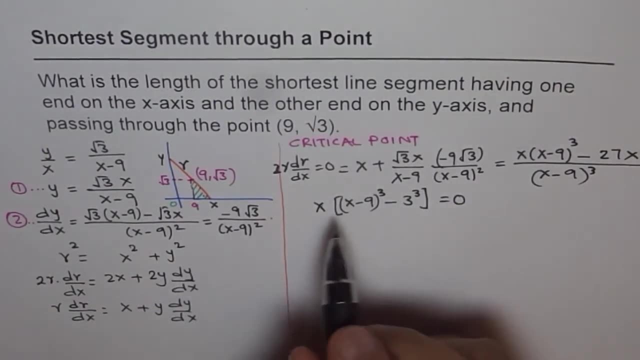 So we get x minus 9, whole cube minus 27,, which is 3 cube equals to 0,. right Now, this is 0 means either x is 0 or this factor is 0. Correct, So that's first. x cannot be 0, because if x is 0, we have a vertical line. 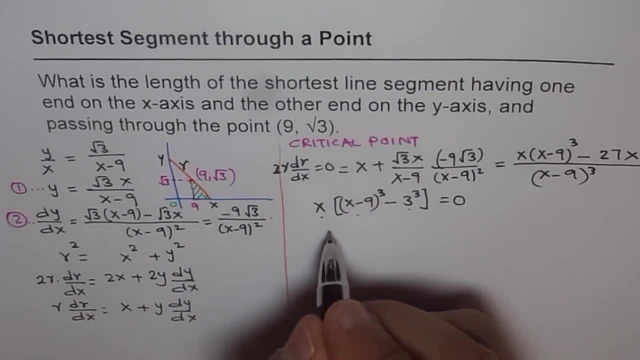 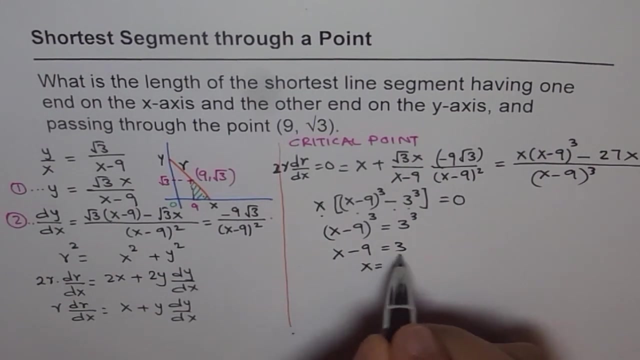 So that is not possible. But well, this could be 0. That means x minus 9, whole cube can be equal to 3 cube. In that case, this factor will be 0. That clearly gives us a solution, as x minus 9 equals to 3, or x equals to 3 plus 9, 12.. 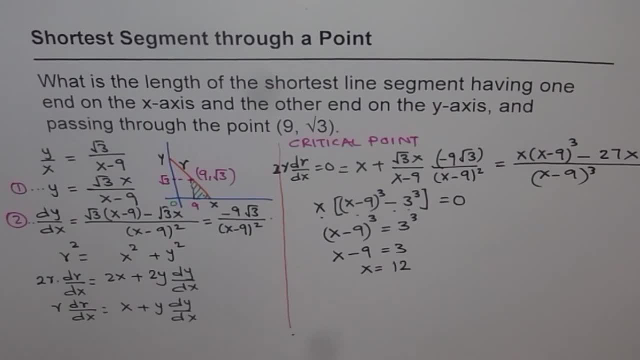 So we do get a solution of x equals to 12.. Now, at x equals to 12, what is the value of y? y is square root 3x over x minus 9.. Let's find that out. So y equals to square root 3x. 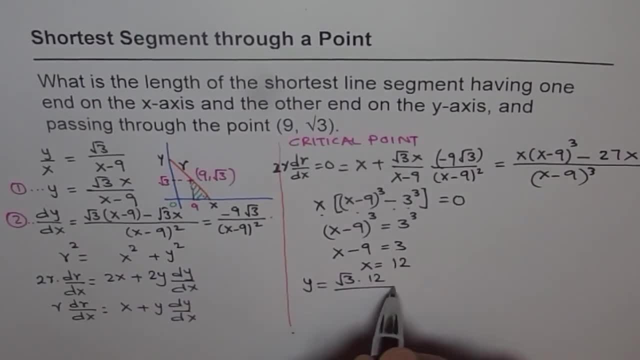 We'll write: square root: 3x is 12 over x minus 9,, which is 12 minus 9, correct, So that gives us: 12 minus 9 is 3, right, So 12 minus 9 is 3.. 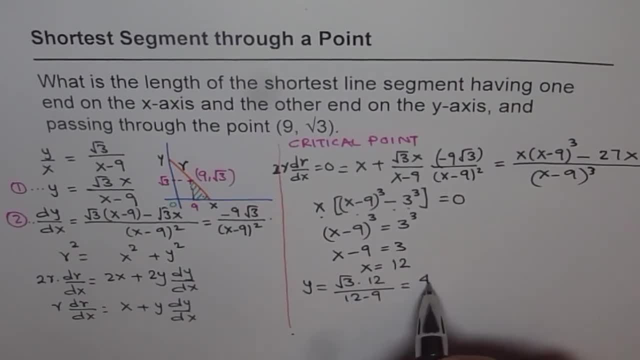 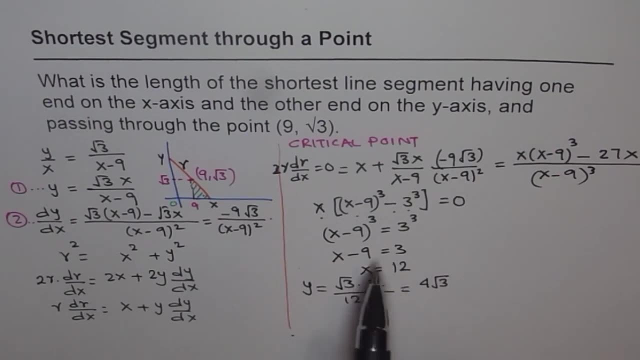 So 3 divided by 12 is 4.. So we get 4.. 4 square root 3.. So that is the value of y. Now for this value of x and this value of y, we can always find the value of r, which is x squared plus y squared square root, right. 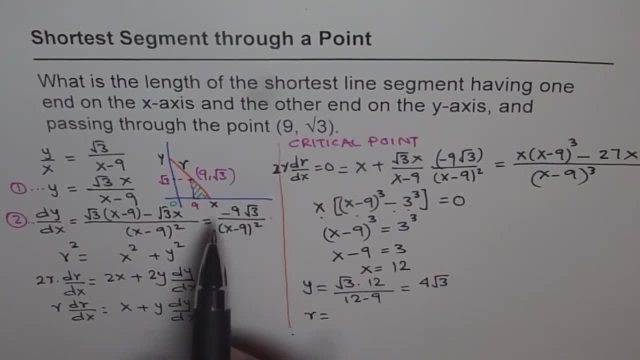 So we have r, which is x squared, which is 12 squared. 12 squared is 144.. Plus y squared, which is 4 square root, 3.. 4 square root is 16, right, 16 times, And this is 3.. 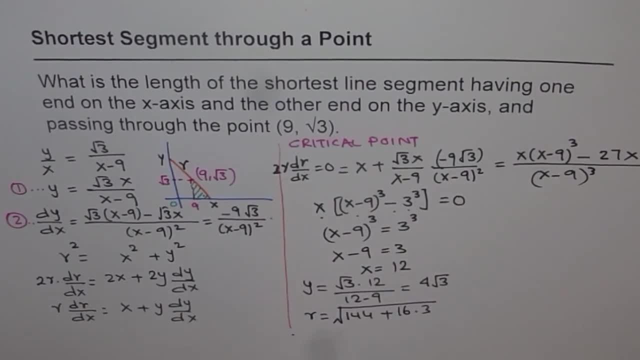 Okay, That is what it is. So 16,. well, 48 I could have written. So that is r. But before getting into this, we know we got a. probably the shortest length is this much? Let's first prove that this is indeed shortest right. 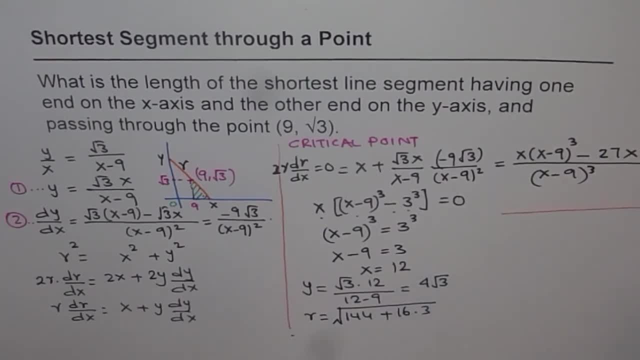 How do we do that? So for that, let's test the derivative itself, that is, dr dx. So what we will do here is we'll test dr dx. We have one critical point, and the critical point is that x equals to 12, right? 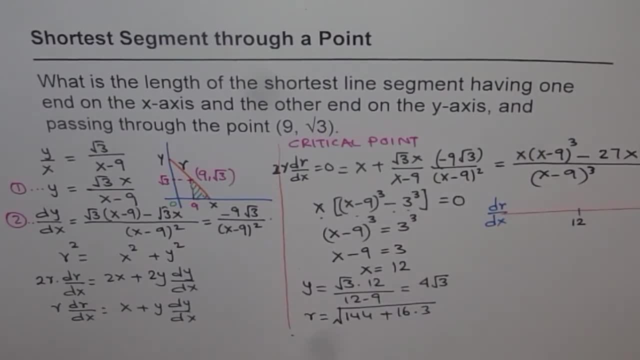 That is a critical point. x equals to 12.. So let us take a test point on either side. So let's say the test point here is 11, and the test point here is 13.. Close enough to 12.. Now that's our derivative. 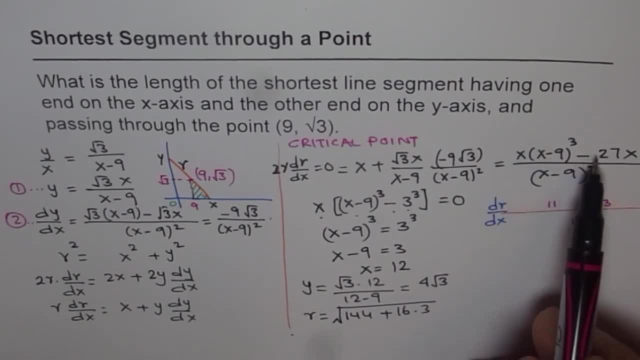 dr dx, is this particular thing Now, which we simplified like that, correct? Now, here you can notice That if I write 11 for x, then 11 minus 9 is 2,, 2 cube And this is 3 cube. 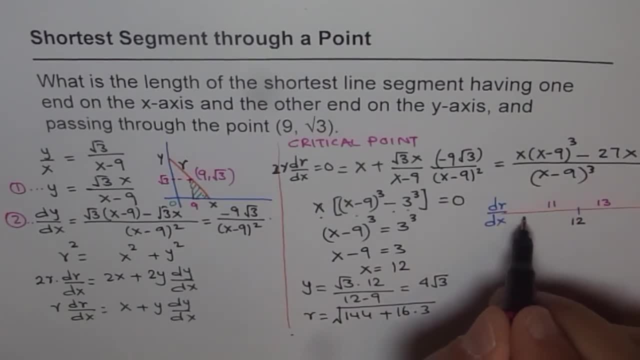 So this gives me a negative value. So we get a negative value. That means it is decreasing, Derivative is decreasing, But if I have 13 here, 13 minus 9 is going to be 4, more than 3.. 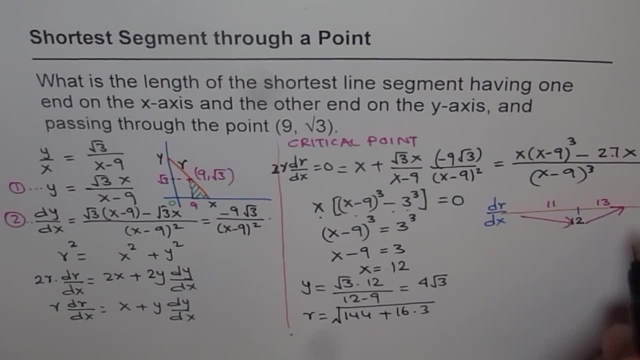 So this will be a positive quantity, So it will be increasing And therefore we see we do have a minimum here, correct? So we have minimum. So we have a minimum at x equals to 12, and we calculated y value as equals to 4 square root 3.. 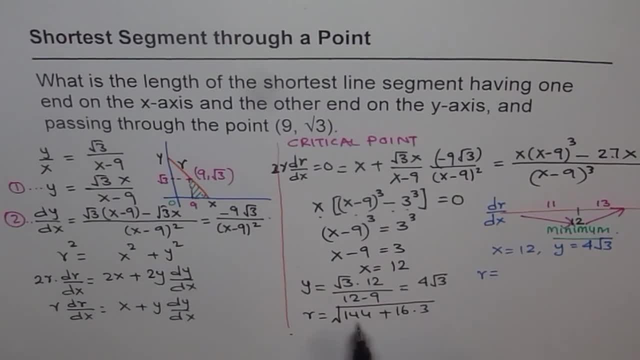 And now we are calculating r, and r is equals to square root of. we have 144, and 16 times 3 is 48.. So 48,. we can add them up right. So So what is that? So 144 plus 48.. 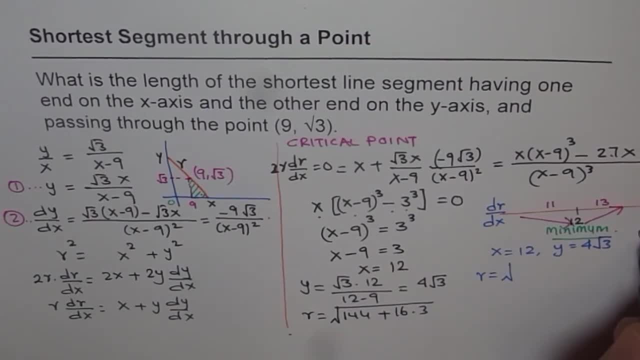 So 8 plus- Let's do this- 144 plus 48.. So 8 plus 4,, 12, and 192.. Yeah, 192.. So we get 192 here correct. So 192 square root is our answer. 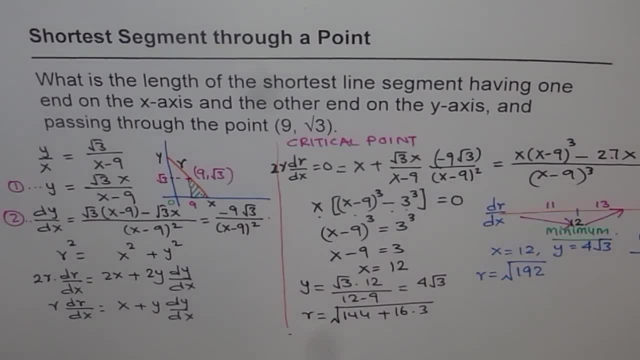 So we can just use a calculator and figure out how much that is So in a calculator, when you put 192 square, What do you get? Square root of 192 is equal to 8 square root 3.. That gives me 8 square root 3, or approximately that's the exact value. 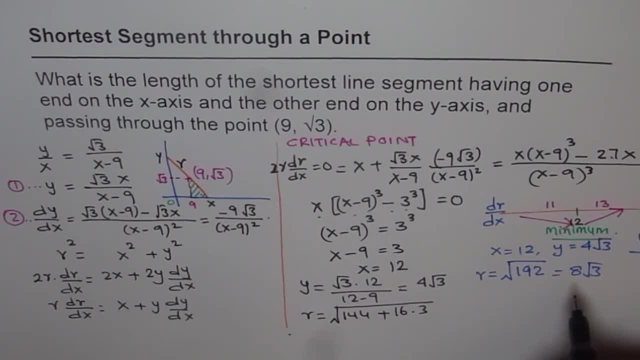 You can change it and get 3.856, 13.856.. So we get 13.856.. We can write 13.856 as approximate value. So that is the value of r which you get Now. this is a very, very important question. 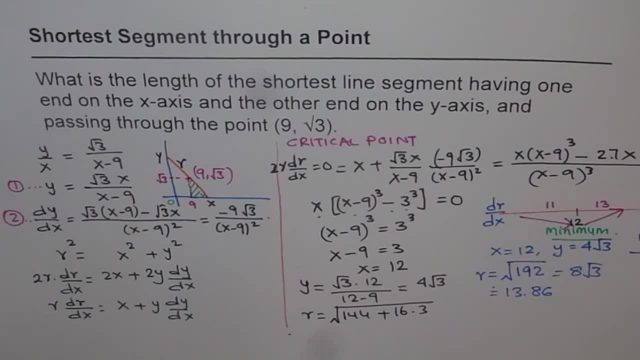 We will see this question A couple of times in different forms, So go through it once again. Remember one thing: that when you have this kind of a situation, you can relate the variables with the help of similar triangles. So that's the strategy used.